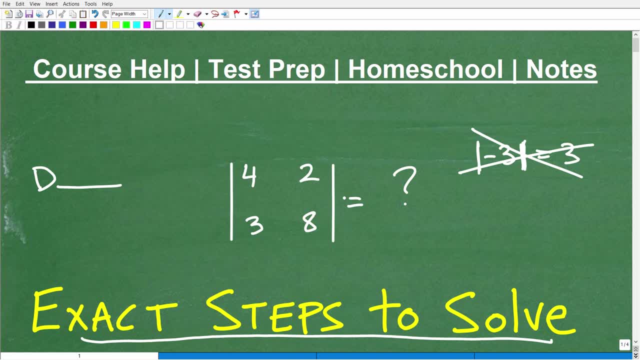 teacher. I'm going to leave a link to my math help program in the description of this video. But if you are having a tough time in math, for whatever reason, okay, maybe you struggle for math, uh, for many years. maybe you hate math, You don't like math, That's okay. But here's the 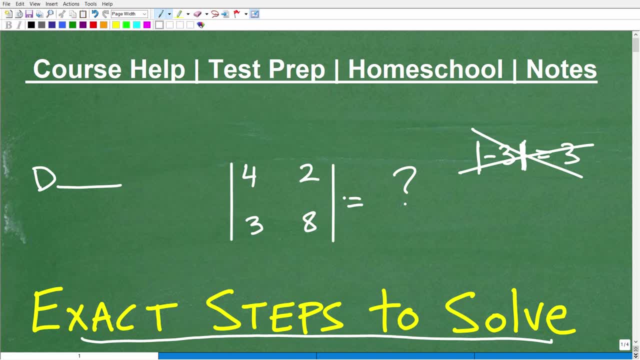 thing. Uh, in order to be successful in anything, you're going to have to change your mindset, And I'm telling you right now, you could be successful in math, and it doesn't have to be so painful, um as well. So, if you're not getting enough instruction in class, maybe not getting 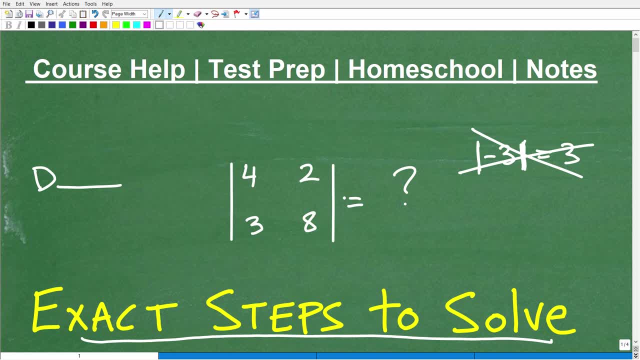 enough time with your teacher, or maybe you're not connecting with your teacher's teaching style. whatever the case might be, I've been teaching math for decades and I really explain things in super easy, clear and understandable. uh, clear and understandable bite size pieces, And that's what you need. You need. 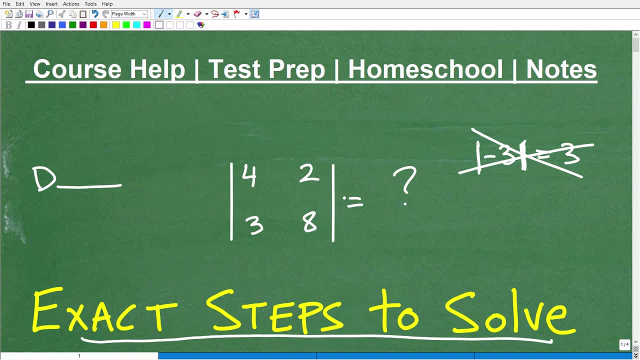 the right instruction. Of course you need to be willing to put in the work as well, But if you had the right instruction and you work hard, you're going to be successful. So if you're at the middle school, high school or college level, definitely check out my math help program If you're having 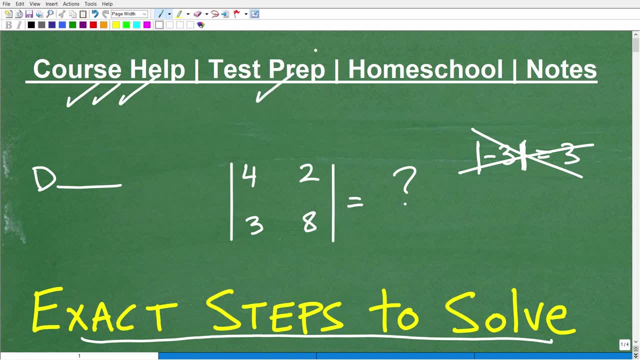 a tough time Now if you're preparing for any kind of test that has a math section and you might not, um, not taking this test right now. you might be taking a test like this in the future. I'm talking about things like: 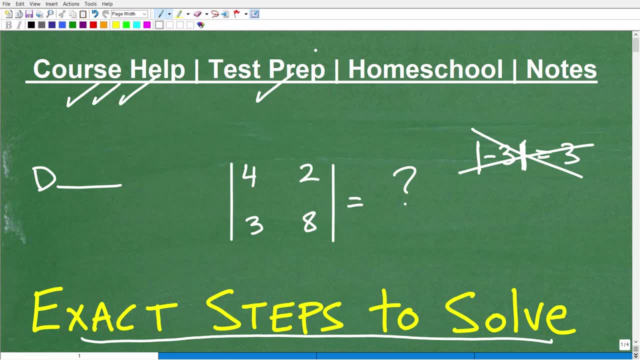 the GED, SAT, ACT, GRE, GMAT, ASVAB, ACMPLACER, CLEP exam, maybe a teacher certification exam. I can help you prepare and pass those exams If you homeschool. you definitely got to check out my. 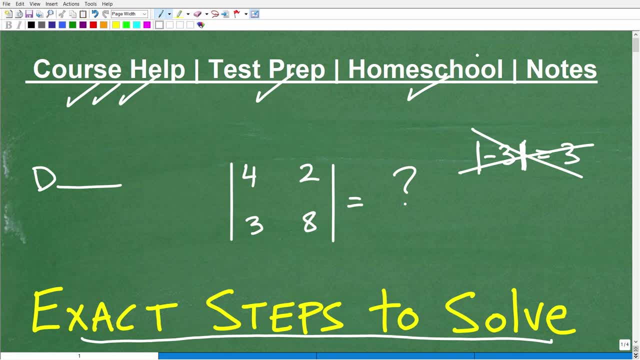 homeschool math courses. They were just voted number one from a big, uh major national homeschool publication, Very proud of that in the category of middle and high school mathematics. And if you need some math notes, I'm going to leave links to my math notes in the description, So if you're, 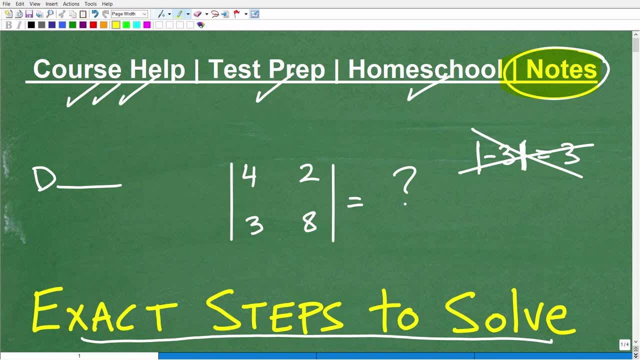 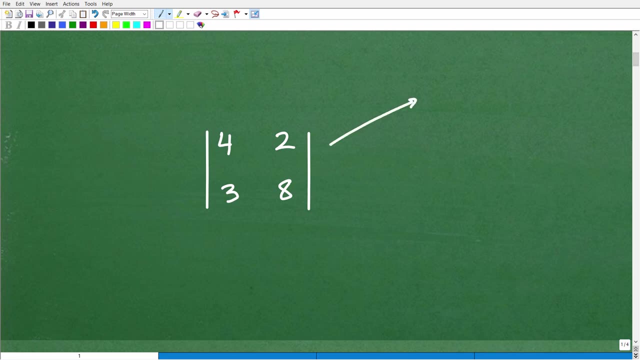 having a tough time in math? the first thing you need to do is start improving your notes. That will help you tremendously. Okay, So let's get into this. So, first of all, before we even talk about, um, how to solve this, what is this? Okay, Like, all right, well, we already talked about. 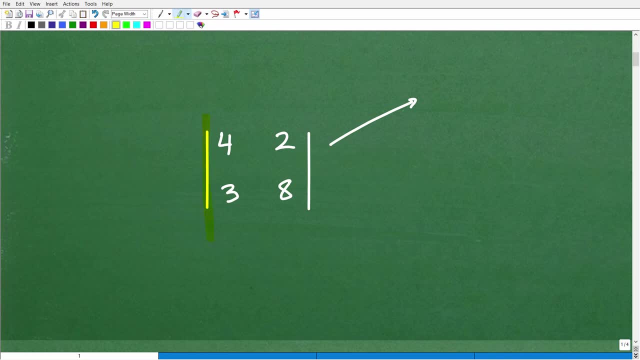 is this absolute value? No, this is an absolute value And in mathematics sometimes we do use the same uh, notation, Uh, you, just you know, but it means something different. Okay, It's just language. You can have the same word that you know. you can use it in various ways: Uh, same. 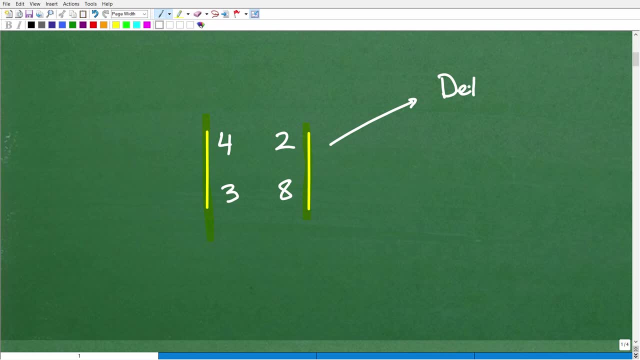 thing in math. So this is a what well, we're talking about a determinant, Okay, But the broader topic here is what well we're really talking about matrices? Okay, A matrix, matrices. So, uh, when you are at the algebra two, college algebra level, you're typically going to, typically going. 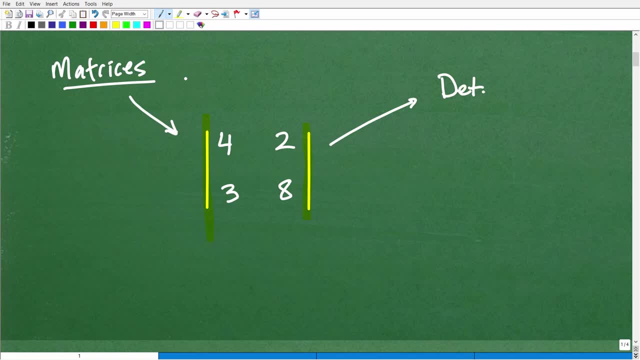 to have a chapter, uh, called something like matrices and determinants, Very, very important. They understand what a matrix is, Okay. So a matrix could be something like four, one, three, eight, seven, nine, Okay, And a matrix- and this is an example of a matrix and just a real quick. 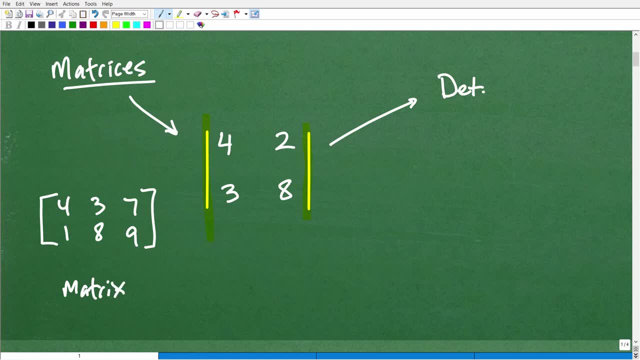 review. It is uh what we would call an array. It's a way to organize information in rows and columns. And uh, let me ask you, uh, in computer programs- and almost 99.9% of you have this on your- 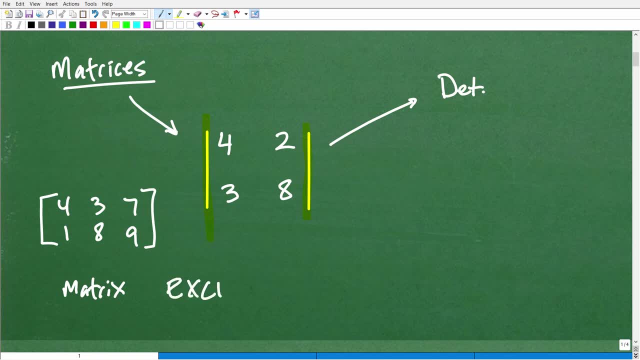 computer, And that is what it's. uh, Excel, right? So if you're familiar with the um software, Excel a spreadsheet. what do you do? Well, you got a bunch of rows and a bunch of columns- the same. 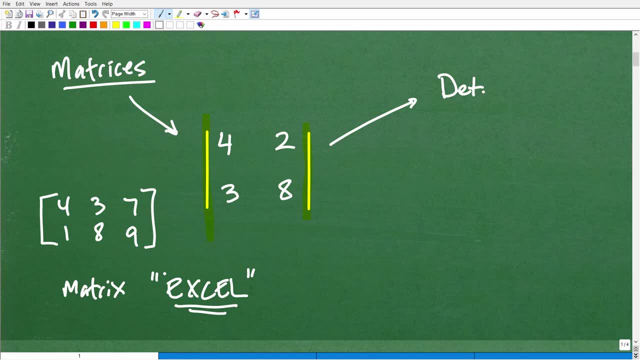 thing, Uh, when we're looking at matrices. that's why um a matrix is so, so, very, very powerful and useful. It's a way to organize um information by rows and columns. So that's a matrix. 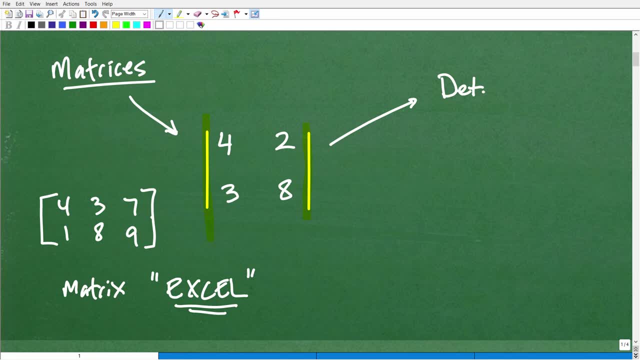 but what do we do with uh? a matrix, Okay, And various matrices? Well, there's a lot of. you need to learn right. You need to know how to add, subtract, multiply, find the uh inverse of. 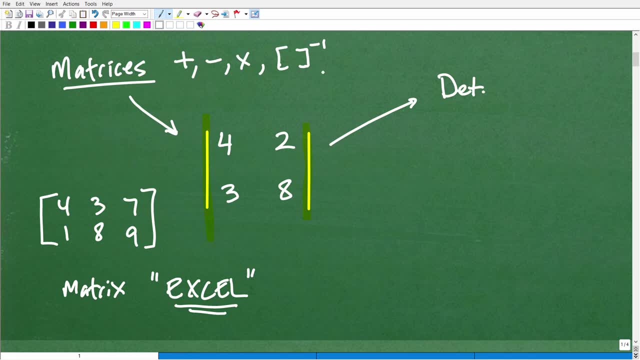 a matrix. Uh, that is a whole nother uh deal. Okay, And uh, what are the other major things you need to understand is how to find the determinant of a matrix. There's a lot of other stuff I'm kind of missing out, but, uh, knowing how to work with matrices, very, very. 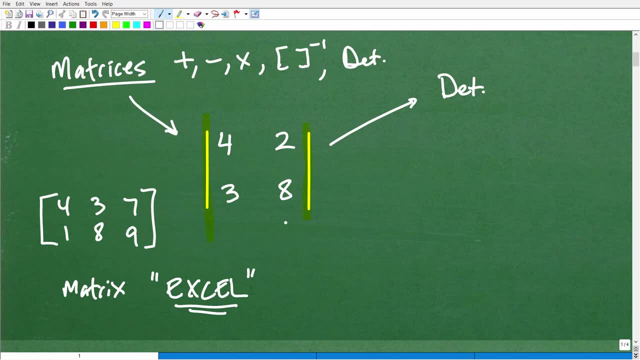 important. So this here, okay, happens to be, uh, the determinant of a two by two matrix, two by two matrix, two rows and two columns. So you can only find the determinant of a, what we call a square, a square matrix, Okay, So in other words, uh, equal number of rows and columns. 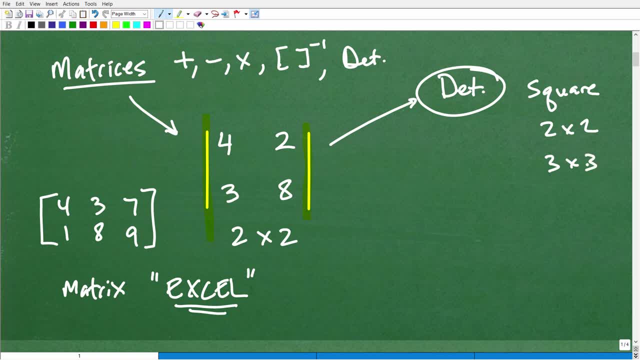 like a two by two and a three by three et cetera. So when you first start learning about determinants, you start learning how to find the determinant of a two by two matrix, to find the uh determinant of a three by three matrix. It's much more involved. So a two by two very easy. 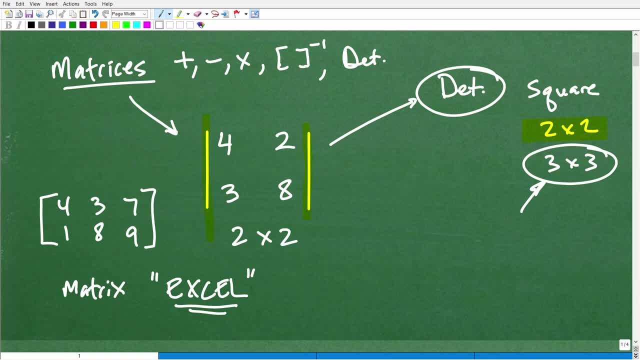 three by three, much more More involved, And there's a couple of different methods to do that. If you're interested in knowing um, how to solve or how to work with um and find the determinants of three by three, 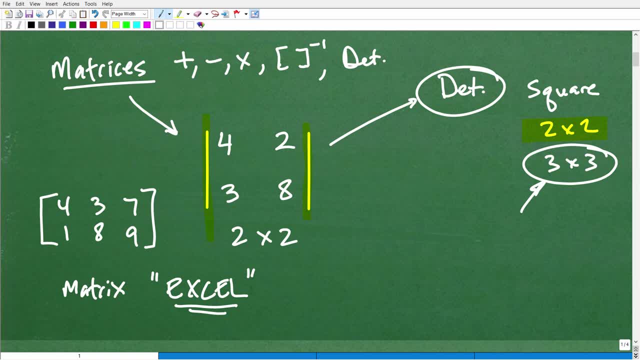 matrices. I believe I have a couple of videos on that on my YouTube channel, but you've really want to thoroughly understand and master all of this. You might want to look at one of my courses, like my algebra two course, my college algebra course or even my pre-calculus course, But uh, 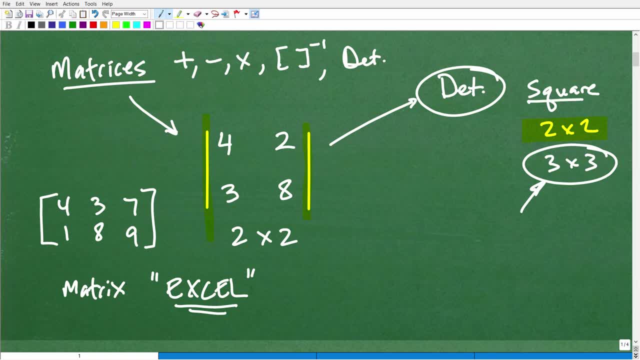 okay. So we're talking about finding the determinant, and we can only find the determinant of square matrices, Okay, IE matrices that have the same number of rows and columns. So if we look at this matrix over here, can we find the determinant of this matrix? Now, this is a matrix. If I wanted to try. 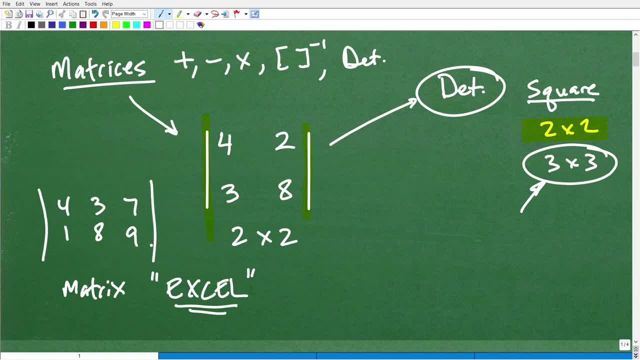 to find the determinant. I would use this notation, right? Unfortunately, this makes no sense because this is not a square matrix. Okay, Uh, this has two rows, Okay, And three columns. So, uh, IE, again, it's not the. the rows do not equal the number of columns, So we can't find the determinant of a. 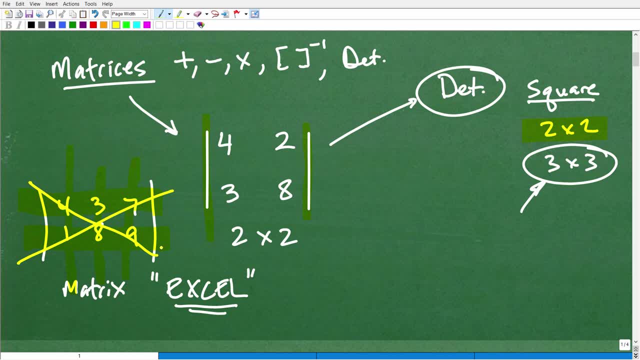 matrix like this. Uh, of course we can do other things with it, like multiply, et cetera, But, uh, again, a determinant is what now? Okay, Well, I already kind of just told you when, when we can. 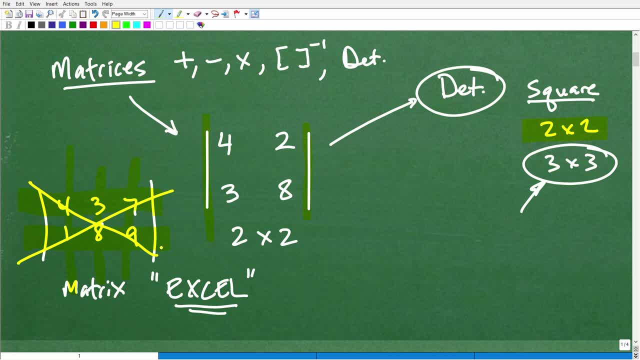 take, uh, the determinant, or when we can find the determinant. but what is the determinant? I haven't answered that question. Well, it's nothing more than a number You're like. well, what does that number mean? Well, it's nothing more than a number. It doesn't mean anything in and of itself, So it's just a. 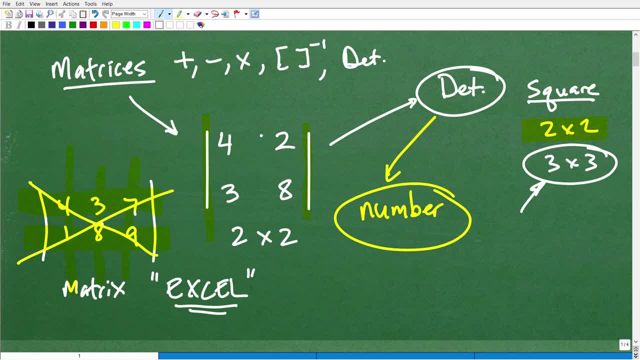 number that's associated with every square matrix. Okay, So the determinant is a number, a value that's associated with every square matrix. However, this number, when we find the determinant, it has a lot of various excellent applications. Okay, It can help us solve other type of problems. 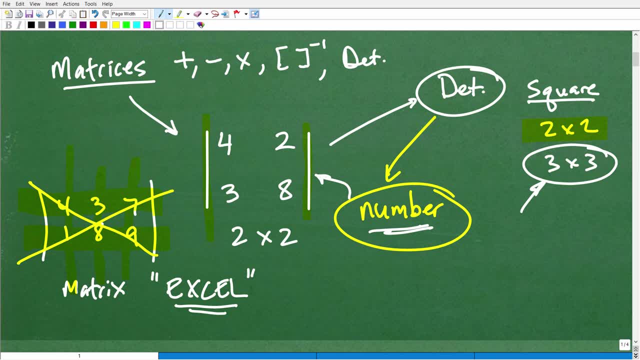 So when we're dealing with matrices and uh, and you can find the determinant, well, you can use that determinant. So, um, but again, the value of the determinant in and of itself is just a number It doesn't have. 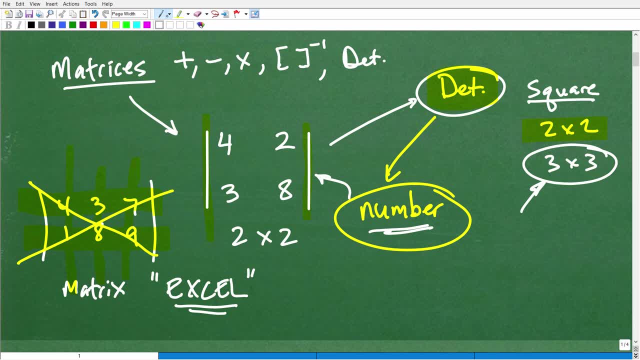 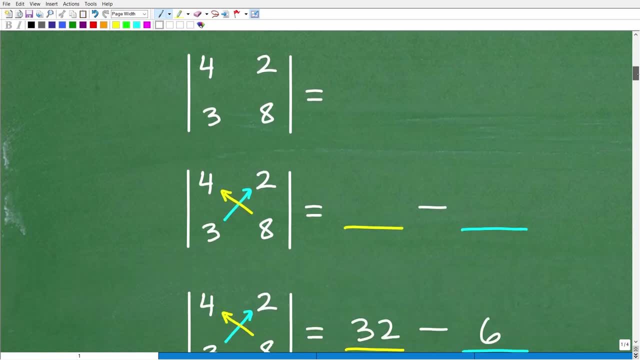 any kind of intrinsic meaning. Okay, So if you knew all that, then that's excellent. Okay, So again. uh, I'm going to get into how to actually calculate the determinant. but it makes no use to calculate the determinant if you don't even know what it is Right? So how do we calculate the? 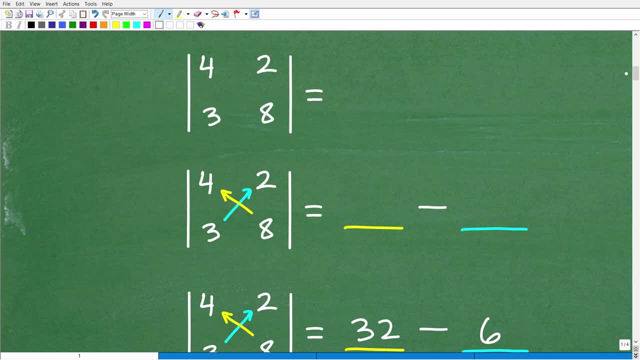 determinant. Well, for a two by two determinant, it is super easy, Okay. So, uh, I'm going to get into how to actually calculate the determinant. Okay, So, what we're going to do, and you have to go in this step, you're going to multiply these diagonals. Okay, So, eight times four, you're. 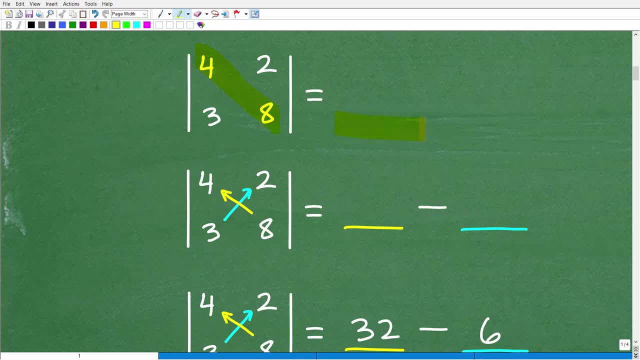 going to multiply this way: first, Okay, You're going to put that answer there, and then you're going to subtract this direction Three times two. you're going to have your answer right there. but you kind of see it, kind of wrote it out this way, So it's going to be, uh, the yellow first. 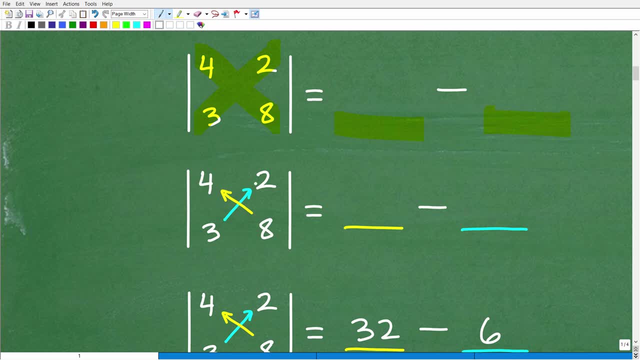 eight times four. It's always this direction, Okay, It's never the other way, It's? you always start with this direction, Okay, So you're going to put that answer there, and then you're going to put this product first. So, eight times four, you're going to put that answer there, And then 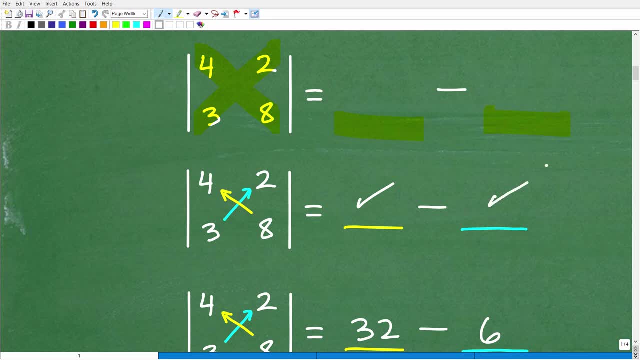 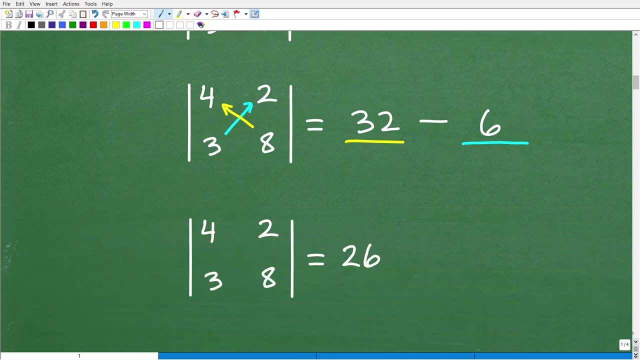 you're going to subtract three times two, You're going to put that answer there. Then the actual value is going to be the determinant. So let's go ahead and see this in action. Again, I told you this was easy to calculate, but the calculating- uh, the calculating- part is not the difficult. 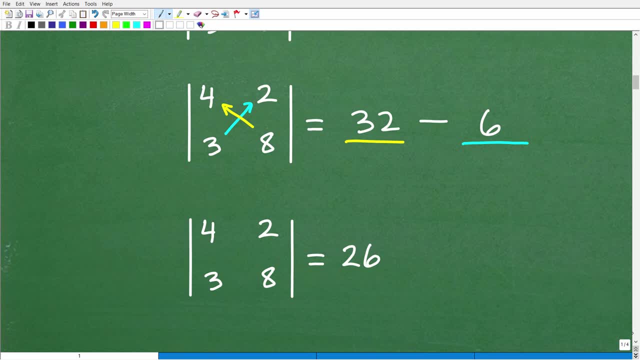 part. Uh, the difficult part is: Hey, what is a determinant, What does it mean, Et cetera. So here we go. So eight times four, of course, is 32, minus three times two is six. Uh, so 32 minus six is 26.. So the determinant of this two by two matrix is 26.. Now again, 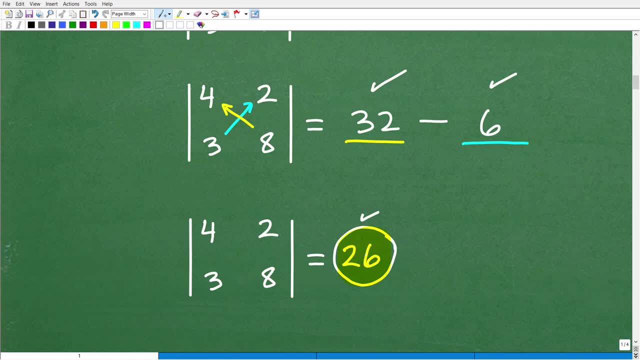 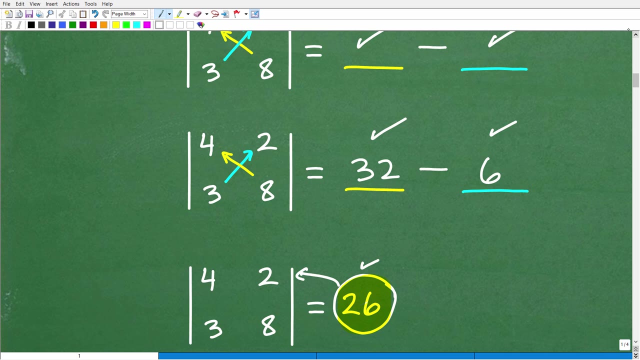 this number doesn't have any value, um, in and of itself. It's just a number that's associated with this square matrix, but we can do things with this in other applications- Okay, Very powerful applications as well. So, uh, one last thing on the determinant of a two by two matrix. If you 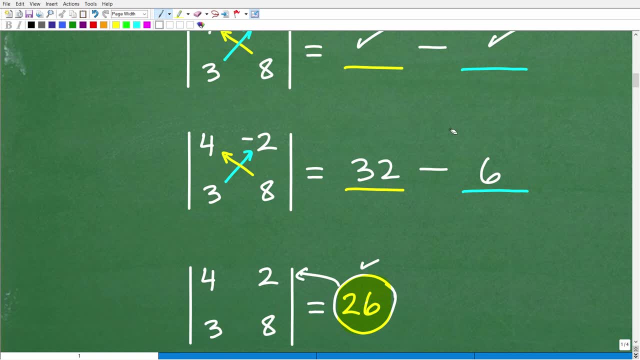 have a negative value. let's kind of change this problem up right here. So let's say I had a negative two as an entry. So I have, uh, eight times four, 32.. Now we have three times a negative two. Let's say I had that situation. You would have to be very careful with that. That's going. 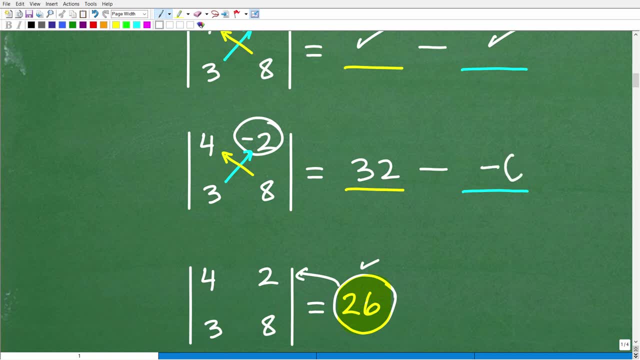 to be negative six. So it's 32 minus a minus six. Okay, Don't make this error. So this is going to be 32 plus six, which, of course, if my math is okay today, it's 38.. So that's another uh uh place where students kind of mess up on these little. 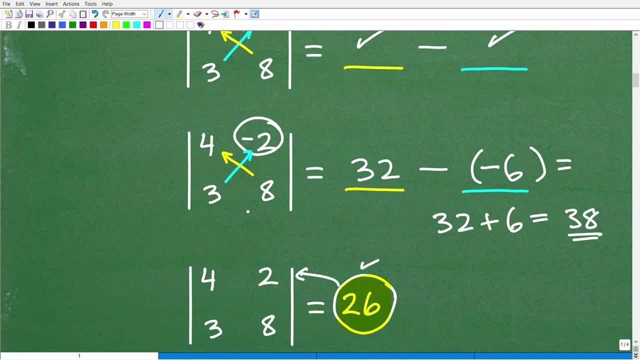 you know negative signs. So be very, very careful. Uh, matrices have a tendency. when you're doing determinants or multiplying matrices- just this whole chapter you're going to see- or as a math teacher for me I've been doing, you know, teaching math for decades. You see all the little bad habits. 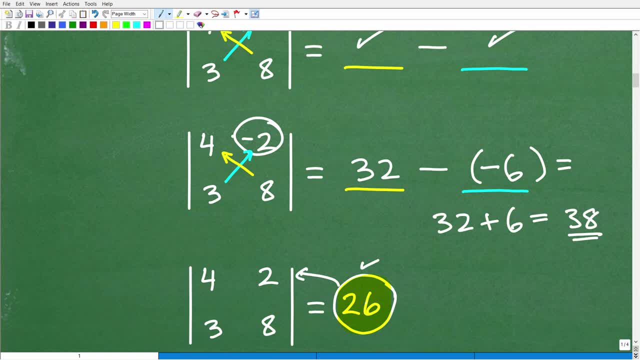 come out with students. If you, if a student hasn't been neat and organized, uh, they're going to make a ton of mistakes because they just kind of uh don't clearly manage. you know, all these little negative signs and positive signs, The 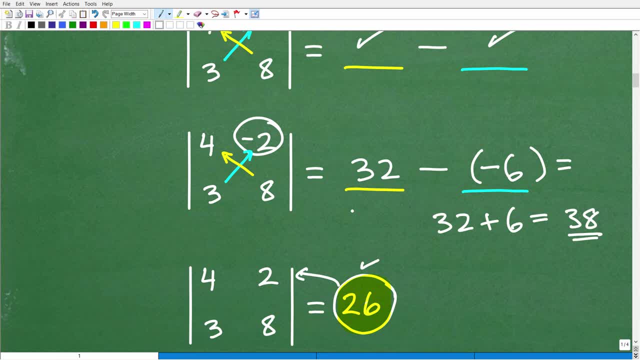 only way you can manage this stuff by is by showing you know, uh, all your work step by step: super clear, nice and neat, double checking as you go. That's how you limit errors. Okay, Anyone's going to make a mistake. If you're doing a lot of math, you're going to make a mistake. I 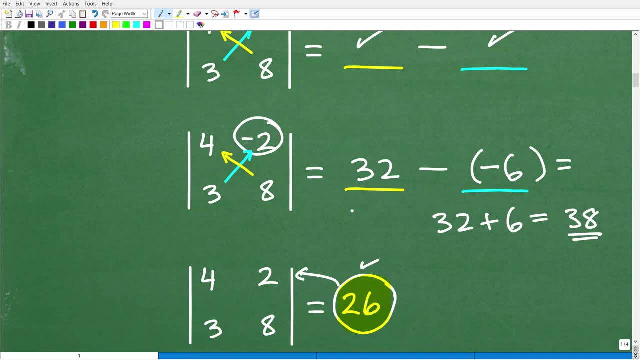 still make mistakes to this day. I try to catch 99.9% of my mistakes, but some of them kind of get through, So that's normal, Okay, Uh, but what you want to do is limit amount of your mistakes, And the only way you can limit your mistakes is one: you got to be super. 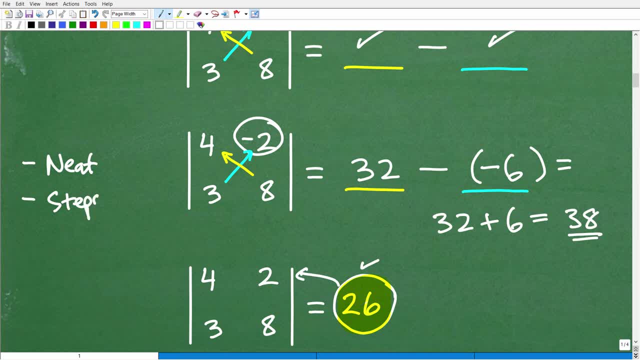 neat too. You got to show your steps, each step, Uh. then you also have to kind of double check as you go. All right, So double check your work, be neat, show your steps, double check. And then, lastly, you got to practice, all right, Uh, and build good um habits in terms of solving uh. 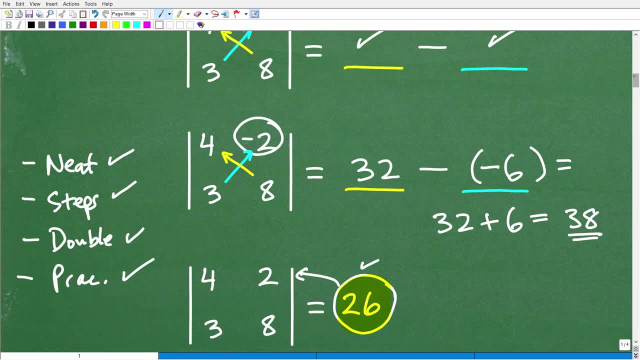 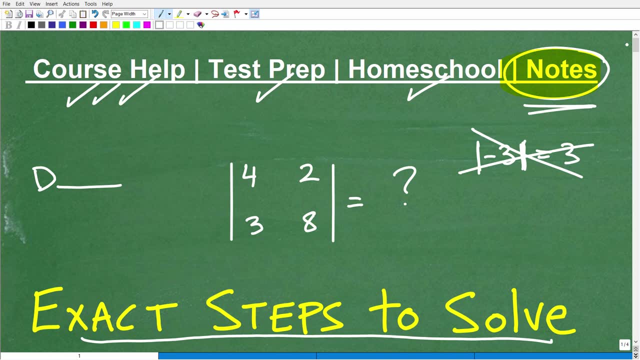 math problems, right? So these steps are universal when we're talking about mathematics. So if you master this stuff, you're going to uh really kind of reduce your uh errors down by 99%, And that's very, very good, right There's.